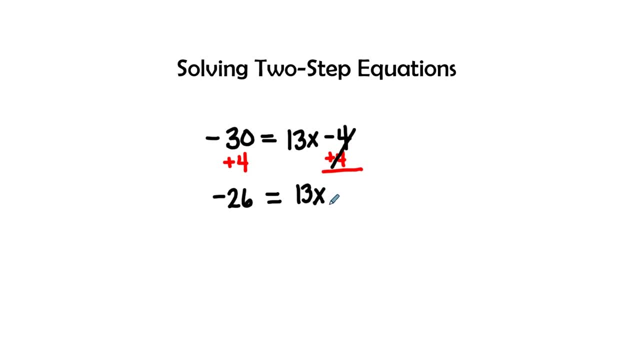 it's with multiplication, So the inverse operation of multiplication is division, And so we're going to go ahead and divide both sides by 13.. Now, 13 divided by 13 is X And negative 26,. and this is a positive 13,. so a negative and a. 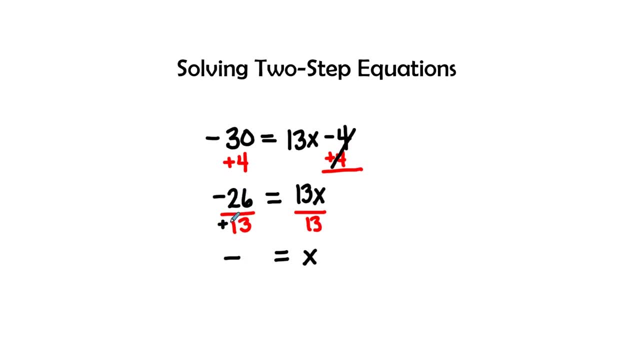 positive gives me a negative answer, And 26 divided by 13 is going to equal 2.. So the correct answer, our answer, is: X equals a negative 2.. Now we can move this into standard form and flip it around, and so we can have X equals X. 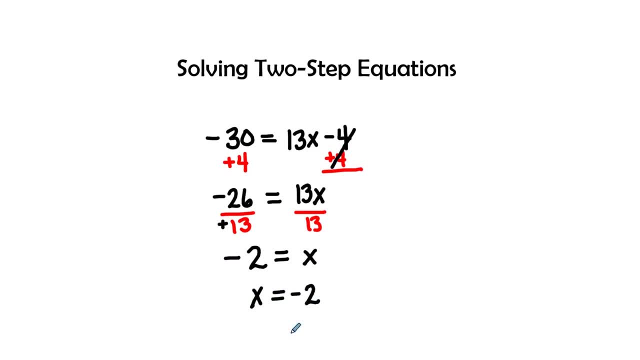 a negative 2.. Now I'm going to go ahead and do this problem a different way. I'm going to rewrite the problem: negative 30 equals 13x minus 4.. And before I get started, I could go ahead and take this entire expression on the right hand side and just move it over to the left hand side. 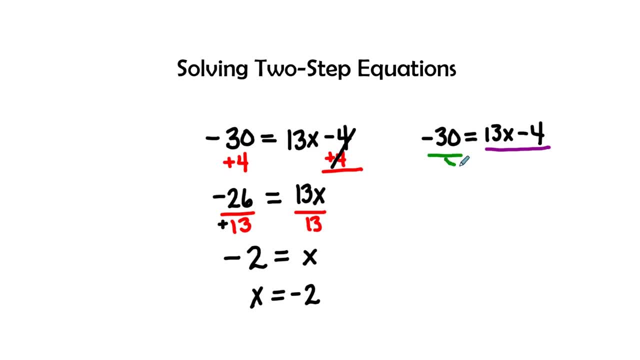 and take this constant of negative 30 and move it over to the right hand side. So let's go show that we're going to move it over. And we have to make sure when we rewrite the equation, that we take every sign along with us. So we'll have 13x minus 4 equals a negative. 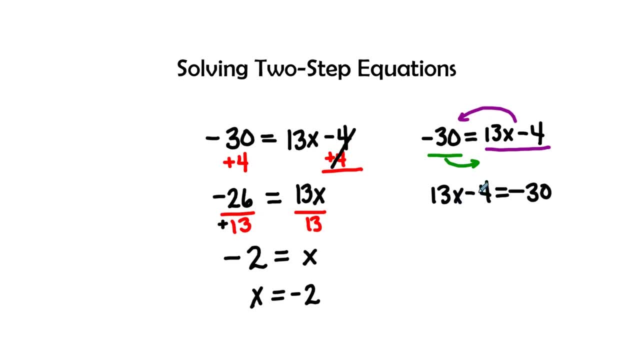 30. So 13x minus 4. equals a negative 30. Now this is a problem that we're used to seeing: All of our variables are on the left and then we have to move anything that's attached. So this negative 4 is attached. So I'm. 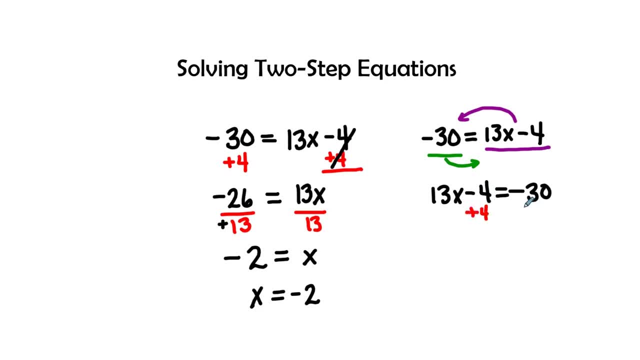 going to go ahead and add its inverse, which is a positive 4, to both sides. This cancels out. We are going to bring our 13x down. Try to keep our equal signs in line. And now this 4,. I should have moved it over in the ones place. So this is negative 30 plus 4,. 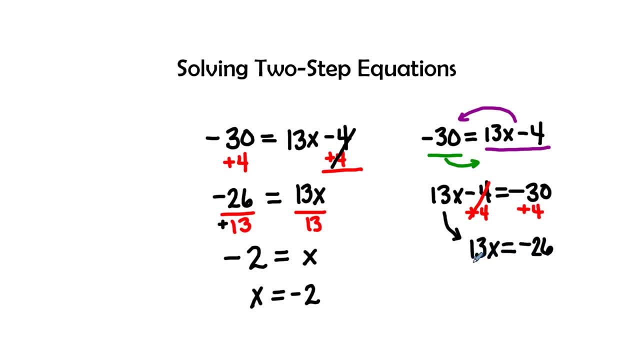 which gives us a negative 26.. We're going to go ahead and divide by our coefficient, which is the 13. It's attached to the x by a multiplication. So we're going to the inverse is going to divide both sides by 13.. 13 divided by 13 gives me x by itself. 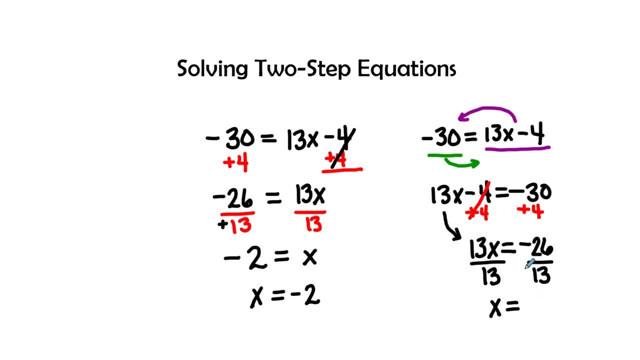 And negative 26.. 26 divided by 13.. Remember, this is a positive, 13. So a negative and a positive is a negative. 26 divided by 13 is 2.. So we do get the same number And as you get more experience, 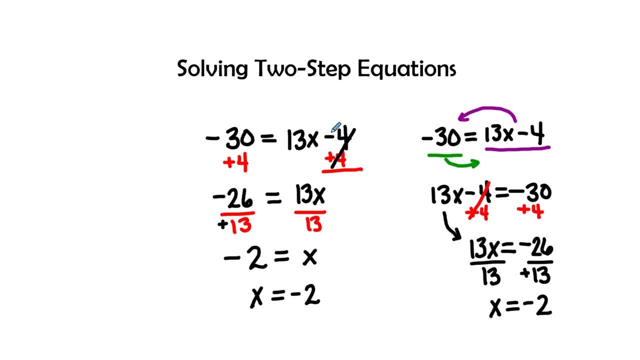 it doesn't matter what side the x value is on, So just keep on working at it. Let's go ahead and check our answers. So I know that I'm going to pull it over here. We're going to do a quick check. 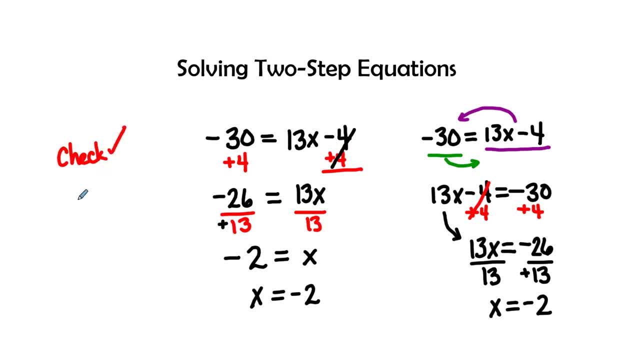 All right, It's always important for us to check. So let's have negative 30 equals 13. And where I see a variable, I'm going to put a parentheses And then, when I add the negative 4, I'm going to insert into the parentheses a negative 2.. 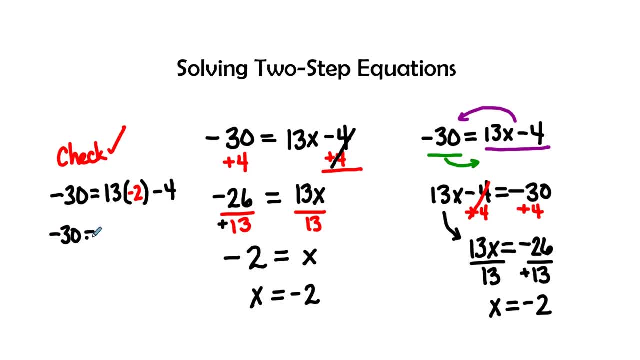 So we have a negative 30 on the left-hand side, 13 times a negative. 2 is a negative 2.. Well, we're going to put a parentheses And then, when I add the negative 2, a negative 26 minus 4.. Negative 30 is going to equal negative 26 and a negative 4.. Now I choose. 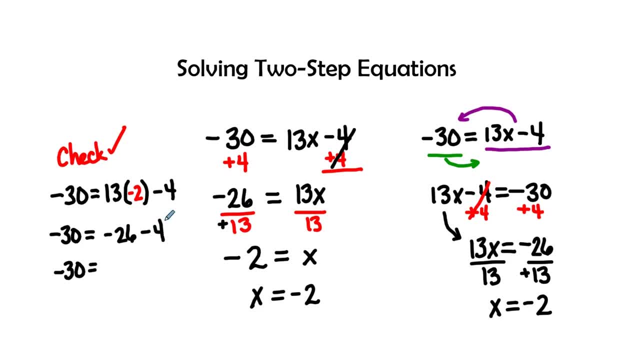 to look at this: when I'm adding integers, I need to keep the sign. I'm going to take the sign before the term, And so this is really a negative 4 and this is really a negative 26.. And then I'm just 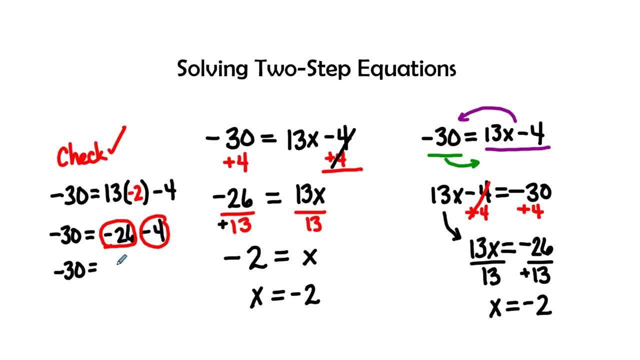 going to add those two together. So negative 26 and a negative 4 gives me that negative 30. So therefore, the answer checks out and I know that I have the correct answer. So remember, in conclusion for today, that it doesn't matter what side the variable is on. I showed you two. 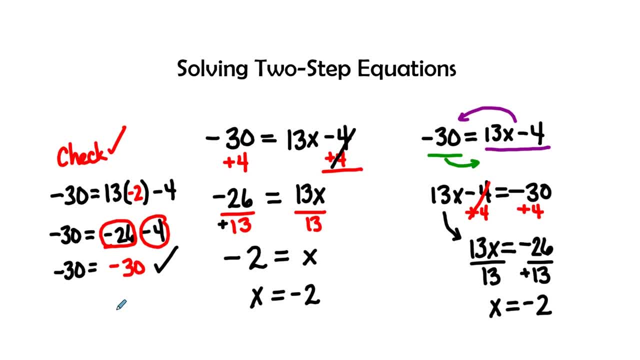 ways today and you pick the one that makes math simple for you. All right, guys, have a good evening and bye. Talk to you soon.